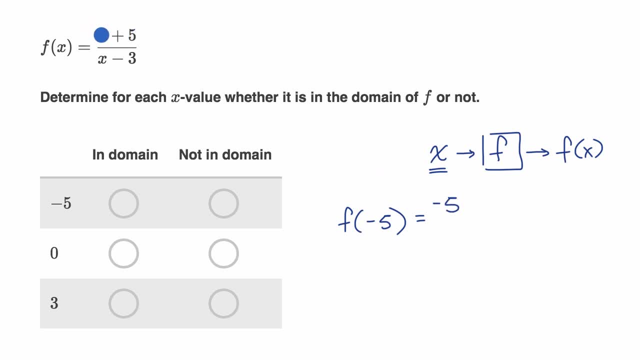 we get negative five plus five. Every place we see an x we replace it with a negative five. So it's negative five plus five over negative five minus three, which is equal to: in our numerator we get zero. in our denominator we get negative eight. 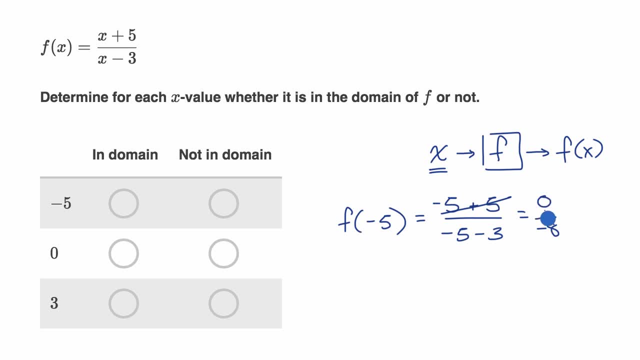 Now, at first you see the zero, you might get a little bit worried, but it's just a zero in the numerator. so this whole thing just evaluates to a zero, which is a completely legitimate output. So x equals negative. five is in the domain. 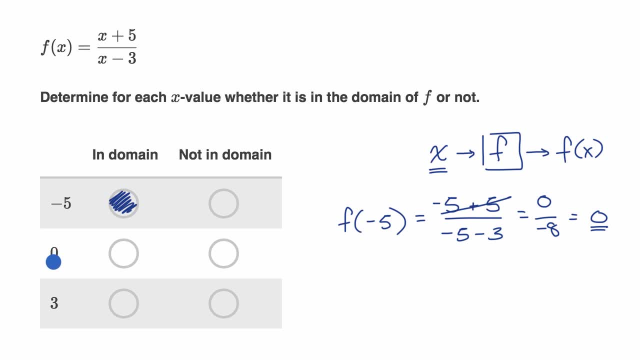 What about? x equals zero? Is that in the domain? Pause the video, see if you can figure that out. Well. Well, f of zero is going to be equal to: in our numerator, we have zero plus five. In our denominator, we have zero minus three. 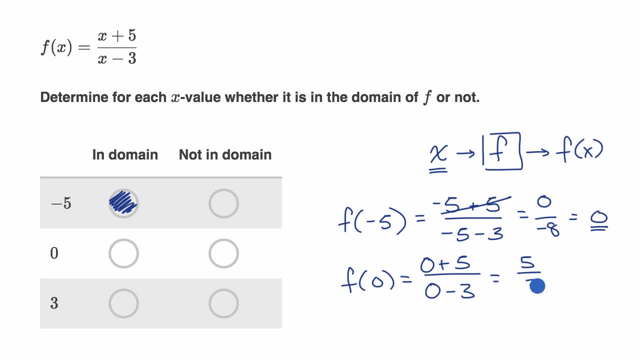 Well, that's just going to get us five in the numerator and negative three in the denominator. this would just be negative 5 3rds, but this is a completely legitimate output. So the function is defined at x equals zero. 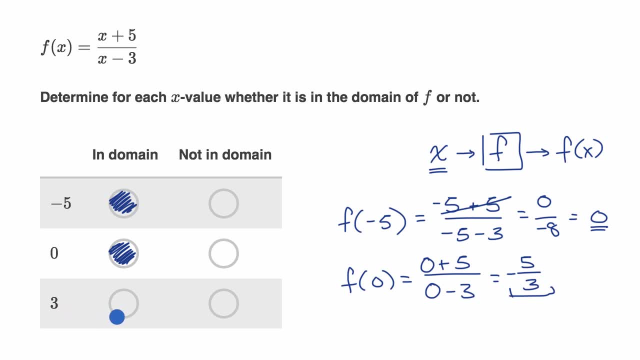 so it's in the domain for sure. Now, what about? x equals three? Pause the video, try to figure that out. Well, I'll do that up here. F of three is going to be equal to what? And you might already see. 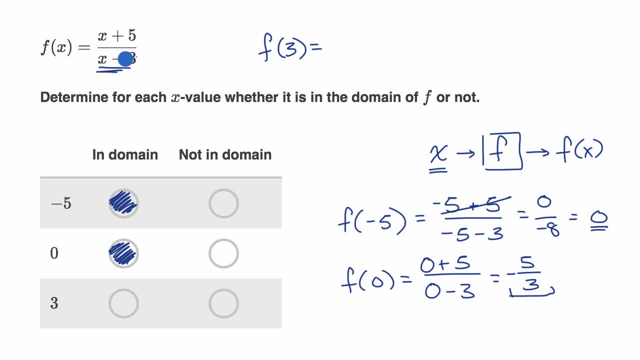 some warning signs as to what's going to happen here in the denominator. but I'll just evaluate the whole thing. In the numerator we get three plus five. In the denominator we get three minus three. So this is going to be equal to eight over zero. 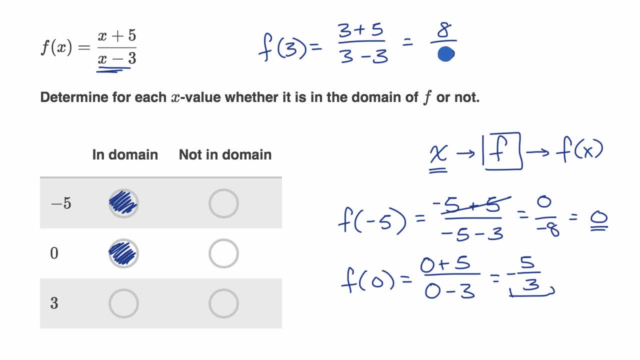 Now, what is eight divided by zero? Well, we don't know. This is one of those fascinating things in mathematics: We haven't defined what happens when something is divided by zero. So three is not in the domain, The function is not defined. 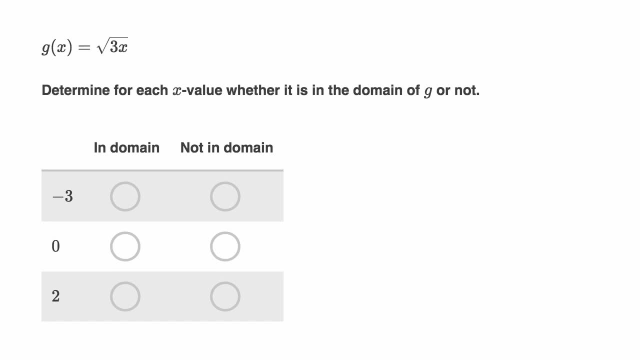 There, not in domain. Let's do another example: Determine for each x value whether it is in the domain of g or not. So pause this video and try to work through all three of these. All right. so first of all, when x equals negative three, 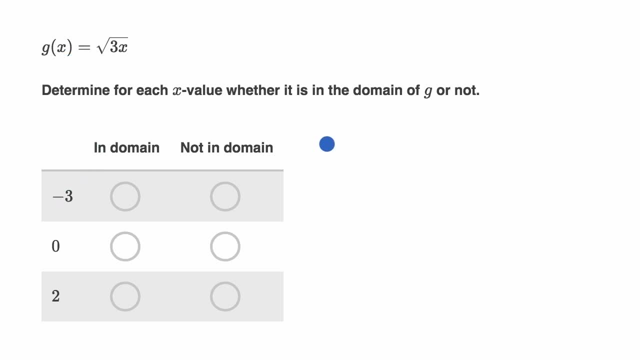 do we get a legitimate g of x? So let's see g of negative three. if we try to evaluate, that's going to be the square root of three times negative three, which is equal to the square root of negative nine. Well, with just a principle square root like this: